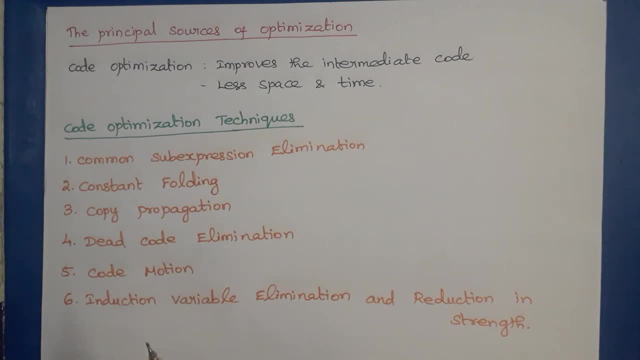 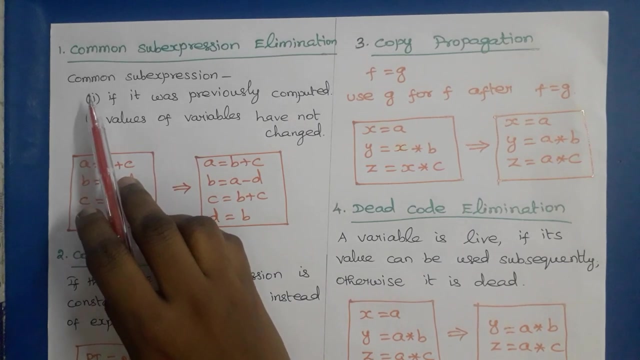 optimization. So these are the properties. One is it should preserve the meaning of the program. Another one is it should reduce the space and time of the running time of the code. So the first one is common sub-expression elimination and expression is called as: 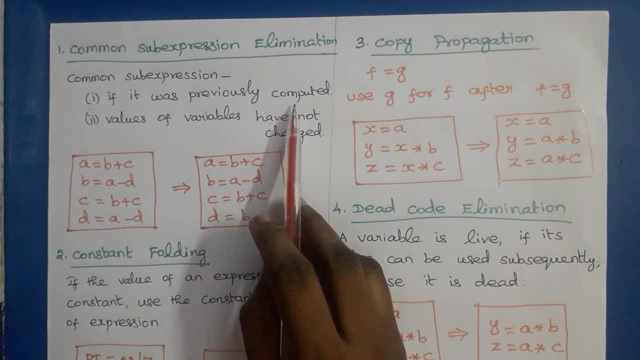 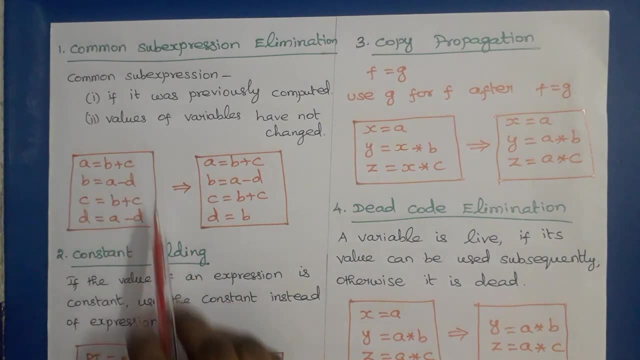 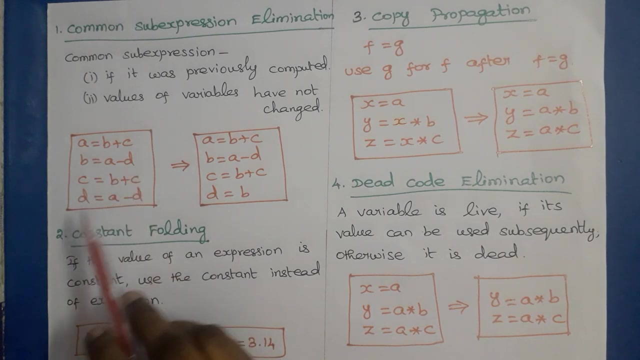 common sub-expression if it was previously computed and the values of variables have not changed from that computation. So for example, consider the sequence of code intermediate code: a equals b plus c, b equals a minus d, c equals b plus c, d equals a minus d. So here b plus c is. 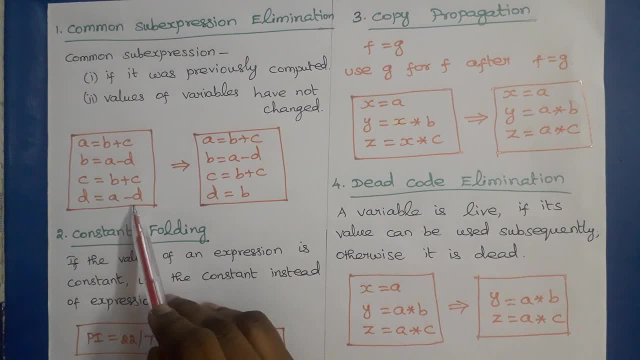 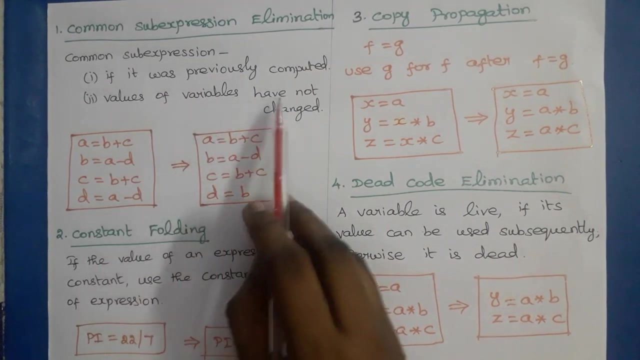 computed two times. b minus d is also computed two times, But b plus c is this third statement. in this third statement, b plus c is not a common sub-expression because the first step it was previously computed, but the values of variables have not changed from this computation right. But here the b is. 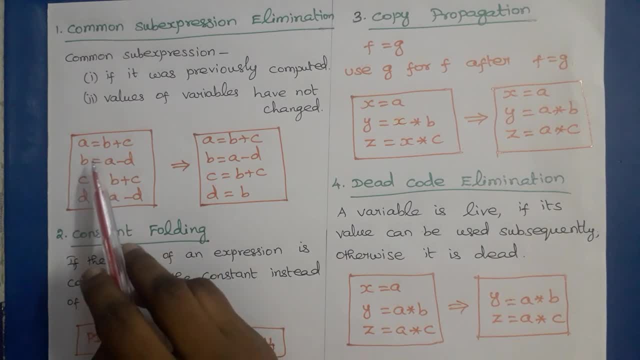 recomputed in the second statement. So the value of b in the first statement is not equal to the third statement. So we cannot say that b plus c is a common sub-expression. okay, So b plus c is not a common sub-expression, but in the 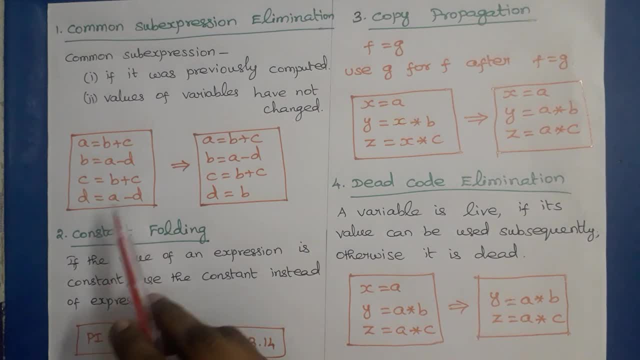 fourth statement: a minus d is called common sub-expression because this a minus d was previously computed in the second statement and the variables a and d are not changed, have not changed from this point. okay, because here a and d is not changed So that we can say that a minus. 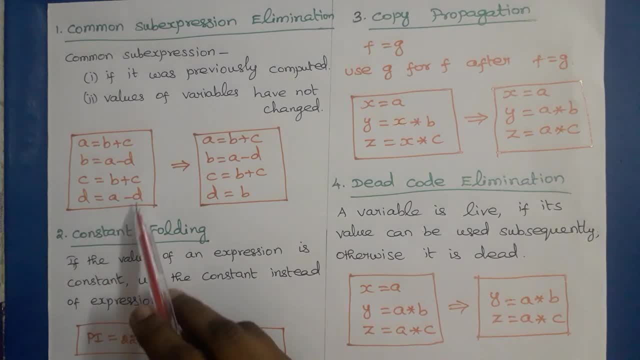 d is a common sub-expression. So instead of recomputing this a minus d again, we can use the b value of variable b here. So we can rewrite that, as this is the optimized code, this is unoptimized code. So after applying common sub-expression elimination, we will get this: 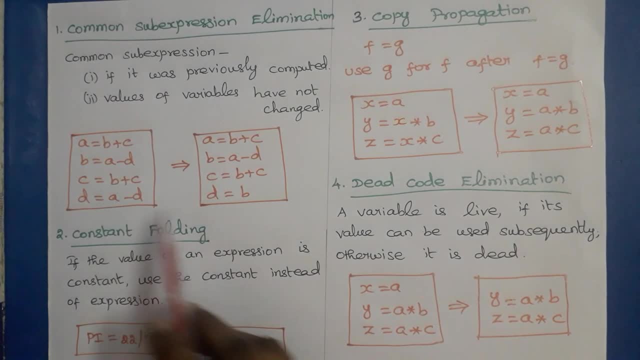 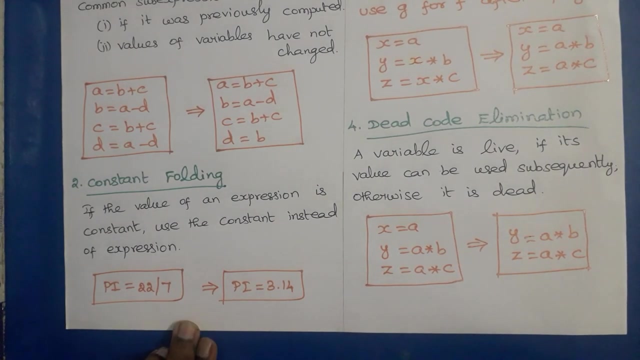 result. So there is no change in first three statements. In the last statement, instead of recomputing a minus d we have to write b, So this is called common sub-expression elimination. Then the second one is constant folding. So this is normally performed at compile time itself. If the value of an 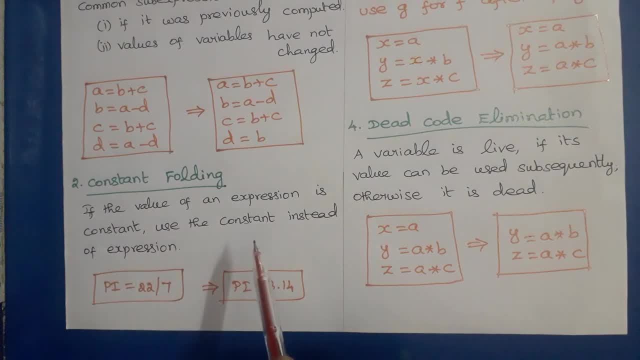 expression is constant, then use that constant instead of the expression. This is called as constant folding. So consider this example here. pi value is equal to 22 bar 7.. 22 divided by 7.. So instead of this one, the result of this expression is a constant right: 22 and 7. both are. 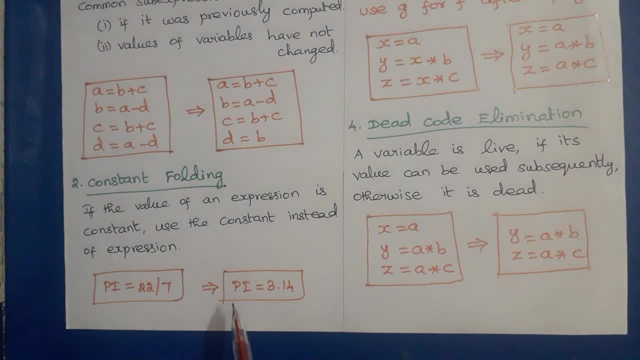 constant. So the result is also constant. So pi is equal to 3.14.. Instead of using this division operation directly, we can substitute 3.14. So this can be performed at compile time. So constant folding means value of the expression. if the value of the expression is constant, use that constant. 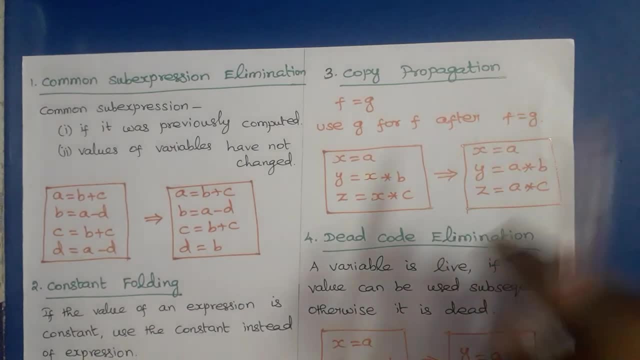 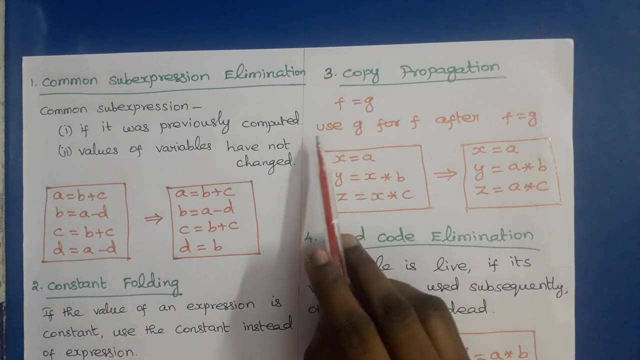 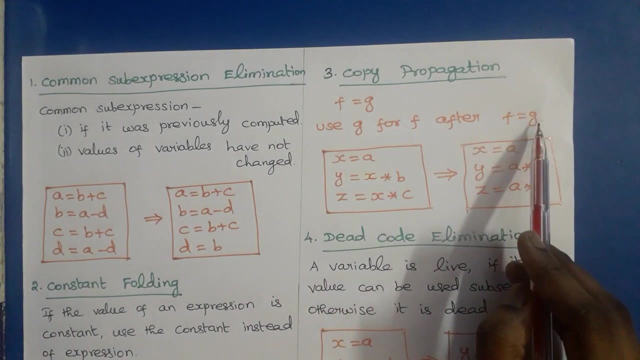 instead of the expression. Third one is copy propagation. So if we have a copy statement like f equals g, then we can use g for f wherever possible after the copy statement f equal to g, That is in this example, x equal to a is a. 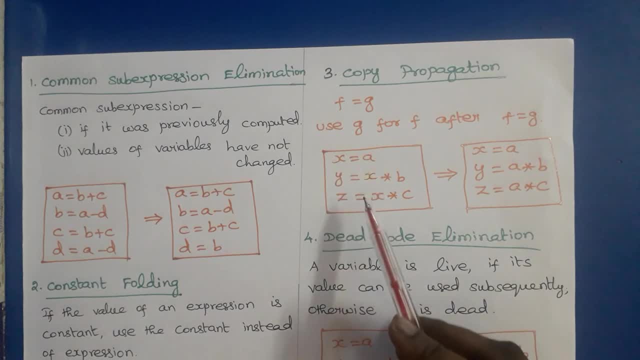 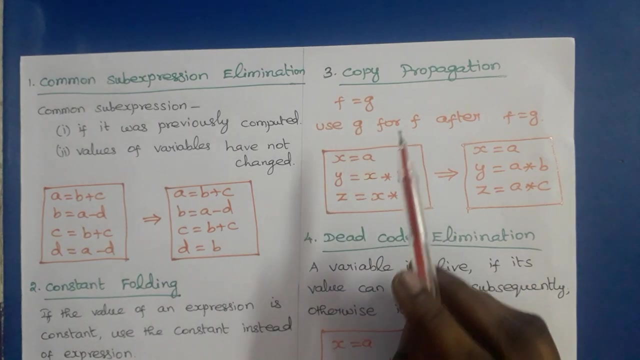 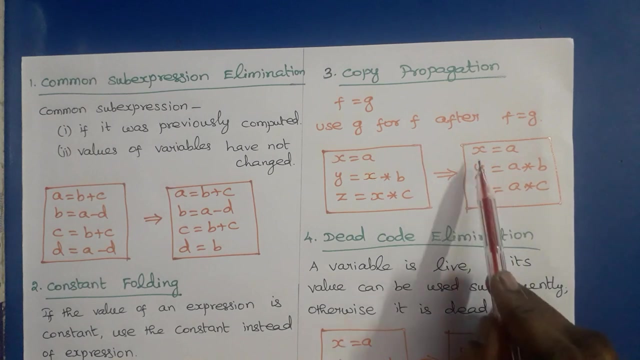 copy statement and in the, in the same block, instead of x in these two lines: instead of x we can use a. That is, if copy statement is there, we need to use the right side of the copy statement instead of left hand side. So instead of x, if you substitute a, we will get this base, this block. So x equal to a. 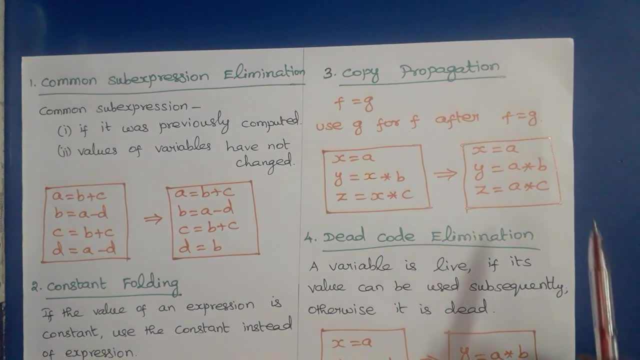 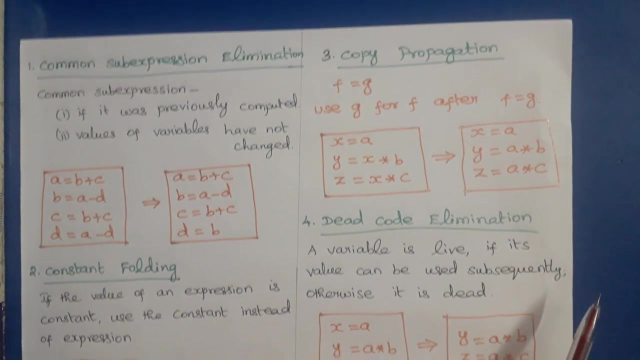 y equals a star b, z equals a star c. So here we didn't see any improvement. Number of statement is also same, but there is a possibility of deleting the x equal to a, So that we can understand from the dead code elimination. So dead code elimination means: 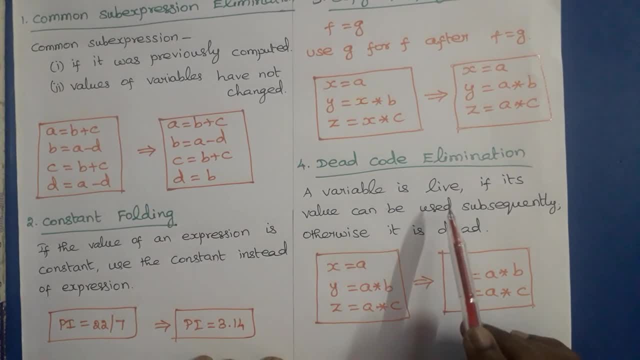 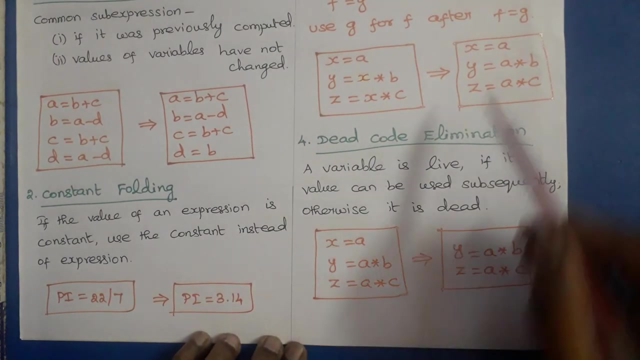 a variable is live. We can say: a variable is live variable if its value can be used subsequently in the program. otherwise it is called as dead variable. So the variable is not live means that is in the same block. we have taken the same block Here. x is not used after. this point means: 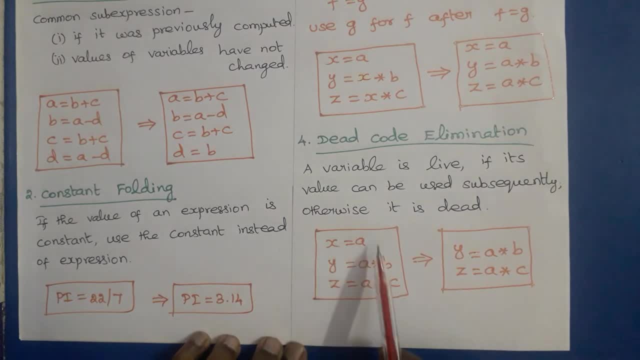 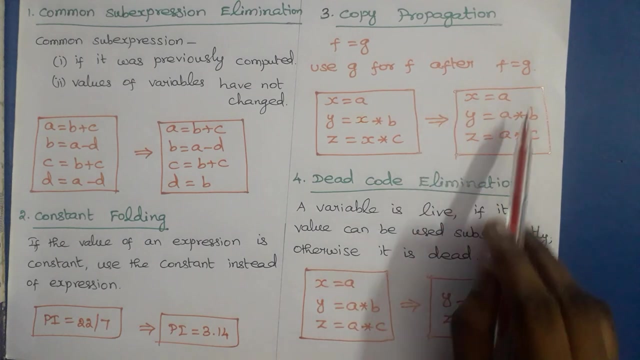 we can say that x is dead. So we can eliminate this copy statement completely Safely. we can remove this copy statement so we can get only two statements in the block. So normally copy propagation will create a dead code, dead variable, So that can be eliminated by using dead code. 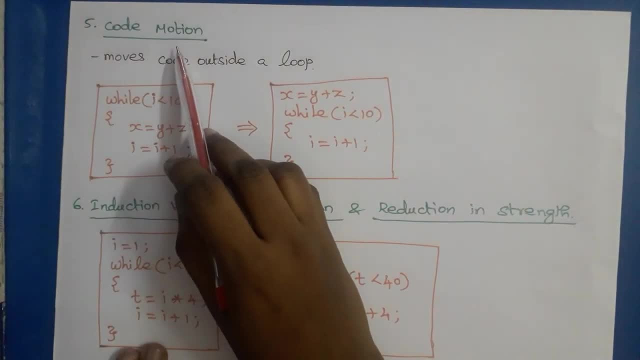 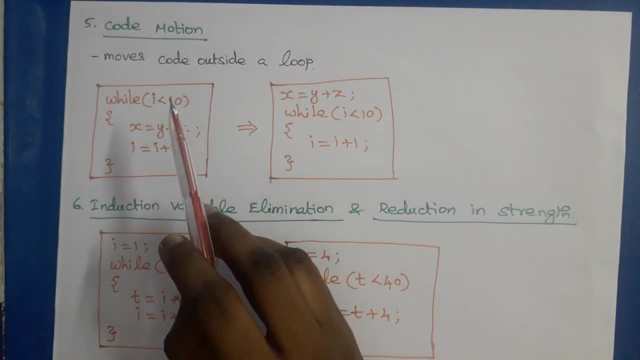 elimination. Next one is code motion. Code motion means it moves code outside a loop. Normally more time is spent for executing the loop, Programs spending more time for executing the loop. So if we move some code outside the loop then we can improve the running time. So, for example, 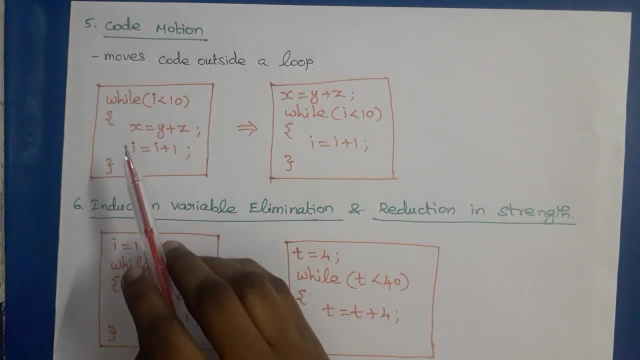 in the statement. and one more thing: if the expression computes the same result independent of number of times the loop is executed, means then only we can move that statement outside the loop. That is, if the expression is loop independent of the number of time the loop is executed. that means that the function is moved outside the loop. undergo the expression Now open the app, be a step information and remove the statement outside of the loop. Therefore, in the state ofrebability, where expression is random, the excitement is valued. So if the expression is conducted in the loop ultimately prevents the result of the state of the output. All in return returns the result of the message exactly outstanding by that. 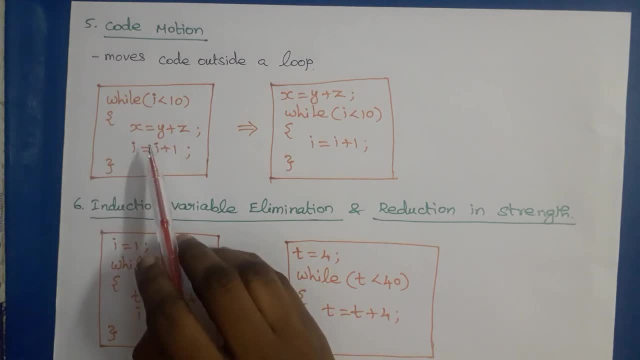 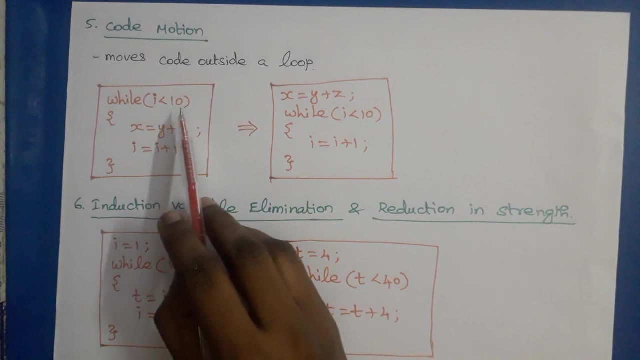 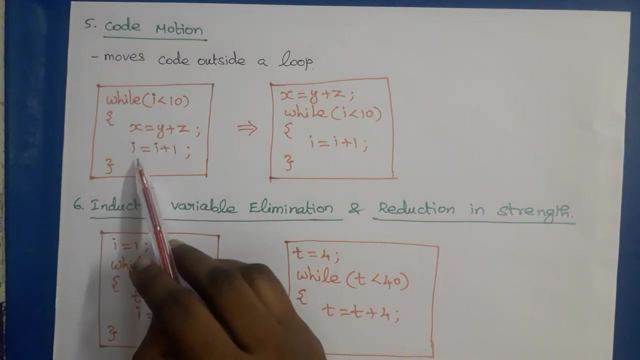 invariant computation. if it is loop invariant computation, then only we can move that expression outside the loop. so in this example, while i is less than 10, two statements are in the body of the loop: x equals y plus z, i equals i plus 1. so this is depending upon. the second statement is: 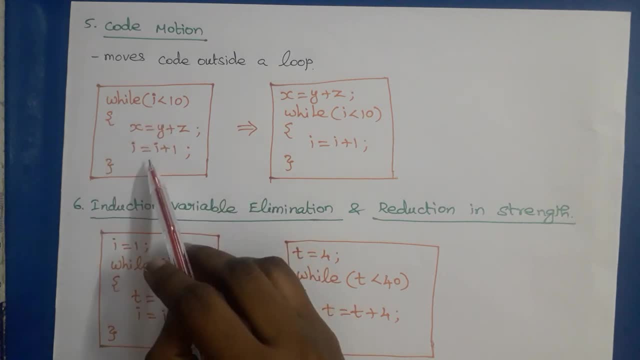 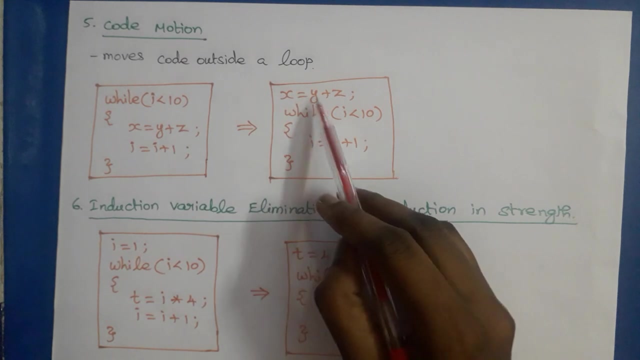 depending upon the loop. so it is based on the loop. so this is not loop invariant computation, but x equals y plus z. it is not based on the loop right, every time x value will be same so that that statement can be moved outside the loop. so if we move this statement outside the loop, 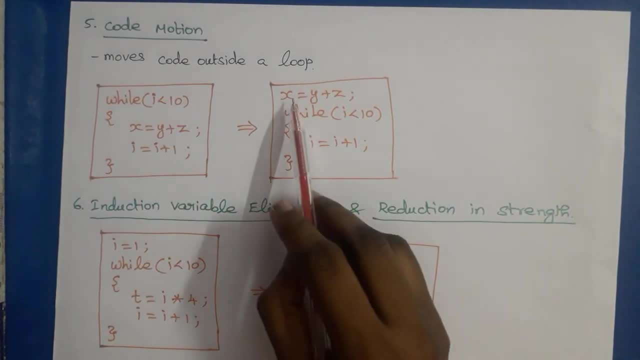 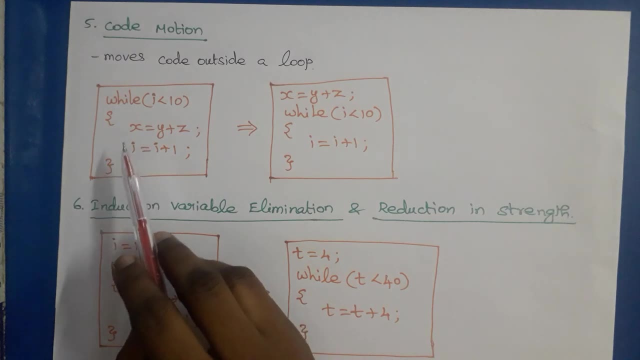 then the number of statement is reduced in inside the loop. so here the statement is executed only once, but in this case this x, equal to y plus z, is executed 10 times, but every time it will give this same result, so that we can move this statement outside the loop. this is called as code motion. 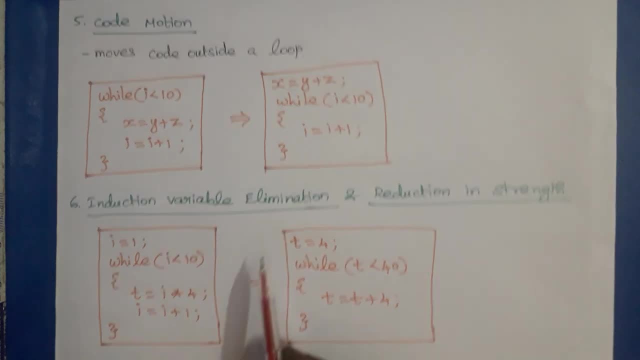 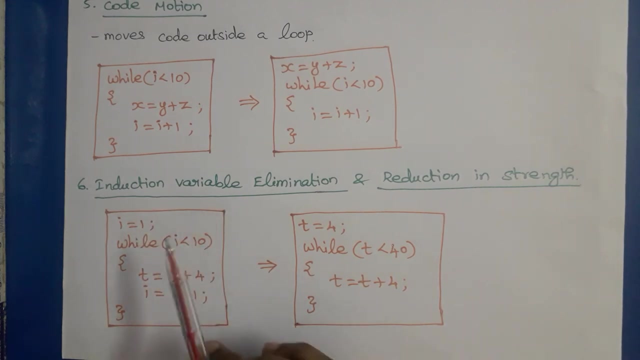 or code movement. the final one is induction variable elimination and reduction in strength. induction variable means it is depending upon the loop loop control variable, like i, j, etc. so that type of induction variable must be eliminated. and reduction in strength. reduction in strength means expensive operations must be replaced by cheaper operation that is complex. 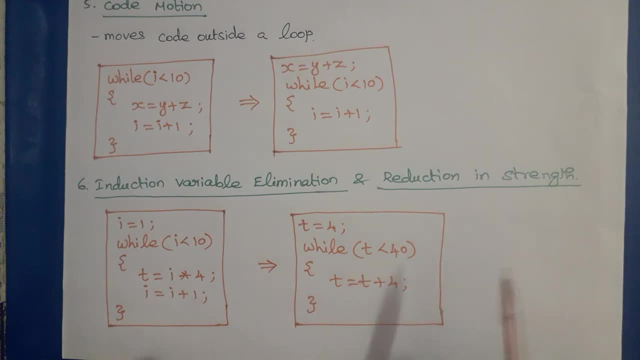 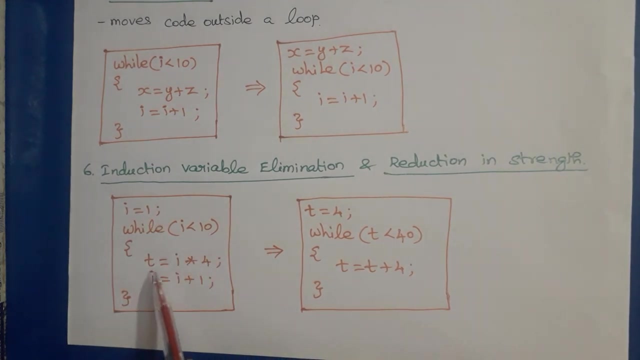 operations must be replaced by the simpler operations. for example, multiplication can be replaced by addition, division can be replaced by multiplication, etc. so in this example i equals 1, while i is less than 10, then t, the variable t is equal to i star 4, and i equals i plus 1. 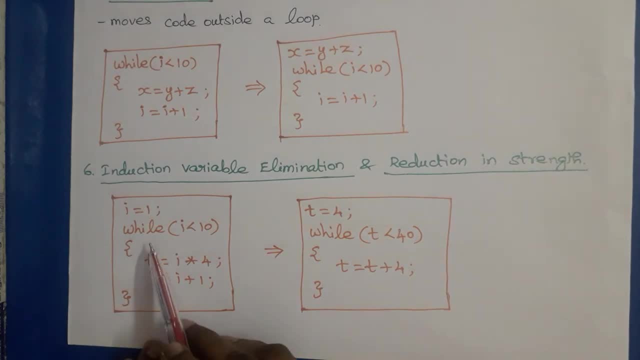 so here this loop is executed 10 times: 1 to 10, so 9 times. the loop is executed 9 times. so each time the t value is increased by 4. right, because initially in the first iteration t is 1, star 4, so the value of t is 4 in the second time, and i is incremented by 1, so 2, 2 is less than 10. 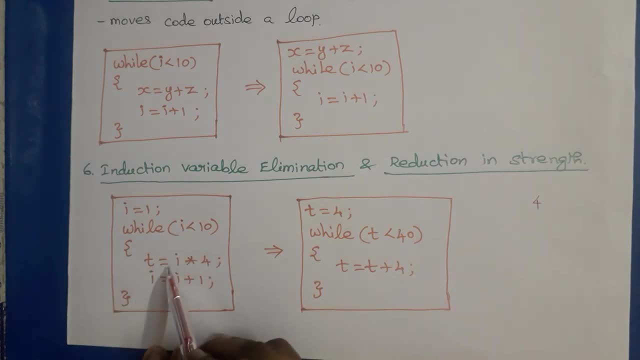 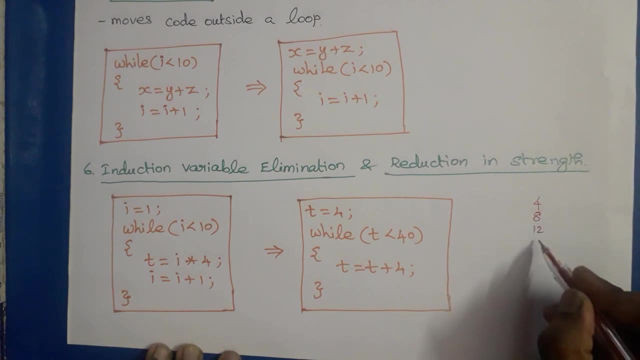 condition is true. so the second time i is incremented by 1, so i is incremented by 2, so i is incremented by 4, and so on, and so on. at the same time t is equal to 2 star 4, so the value of t is 8. then i is incremented by 1, so the value of t will be 12, 16, etc. so at each iteration, 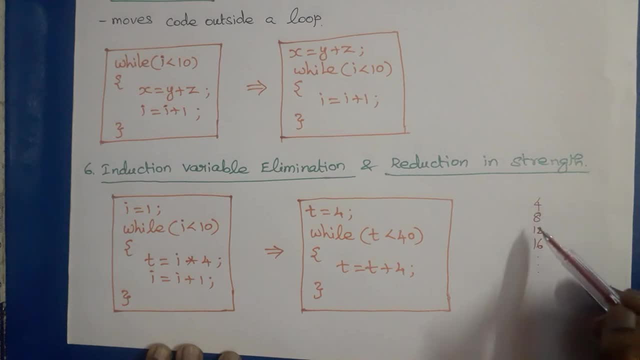 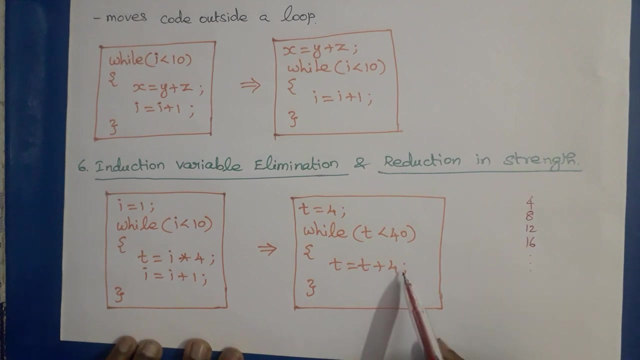 the value of t is increased by 4, right. so this multiplication can be replaced by addition, so reduction in strength can be performed. then induction variable i can also be removed. okay, in the optimized code, that is, instead of t equals i, star 4, we can write t equals t plus 4, right?